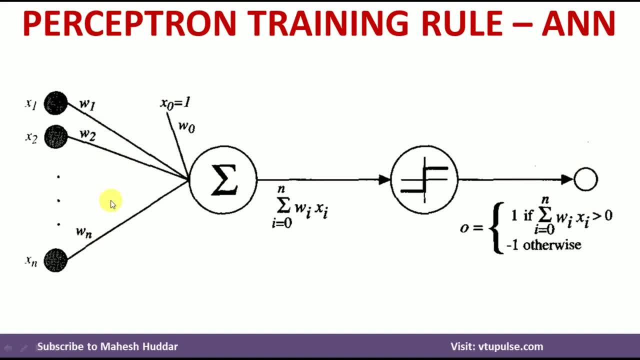 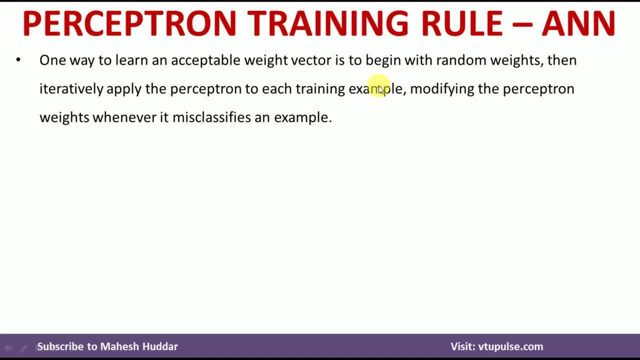 weights. Now, how to learn this particular weights, that's the next question Here. one way to learn the acceptable weight vector is to begin with a random weights, then iteratively apply the perceptron to each training example. modify that perceptron weights whenever it misclassifies an example. 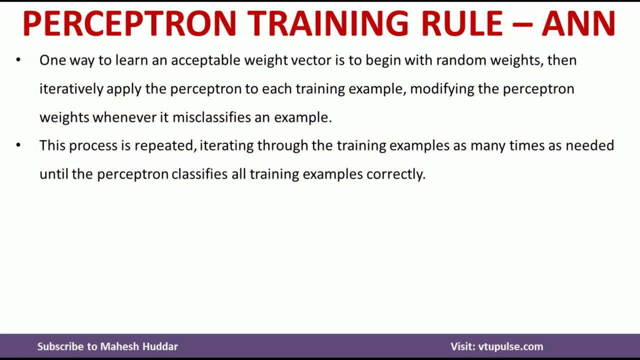 This process is repeated, iterating through the training examples as many times as needed until the perceptron classifies all the training examples correctly. The weights are modified at each step according to the perceptron training rule, which revises the weight wi associated with input xi according to the following rule: 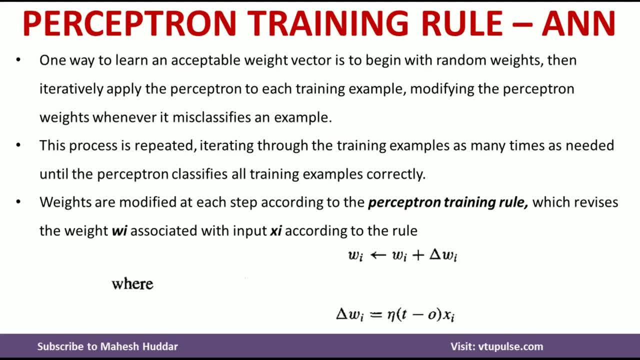 That is, wi is equivalent to wi plus delta, wi delta wi is equivalent to n into t minus o, xi, Where n is the learning rate, which is set to a small value like 0.1.. T is the target output and o is the actual output and xi is the input associated with. 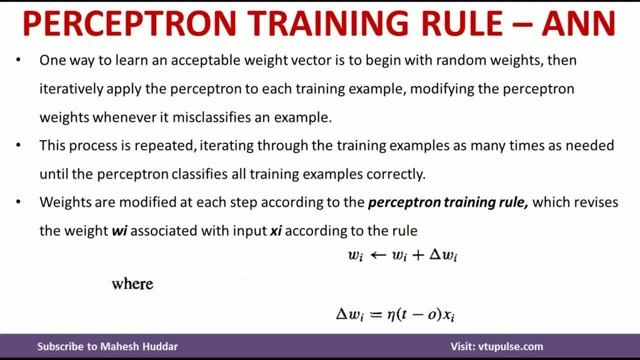 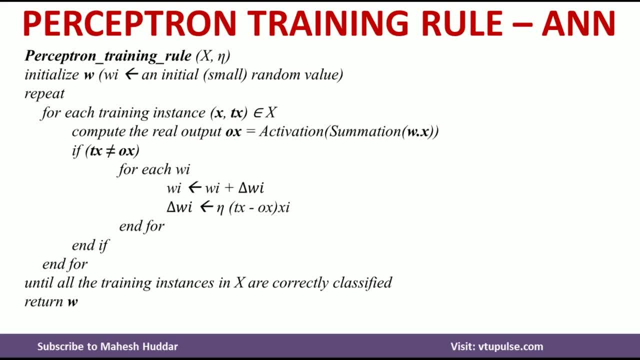 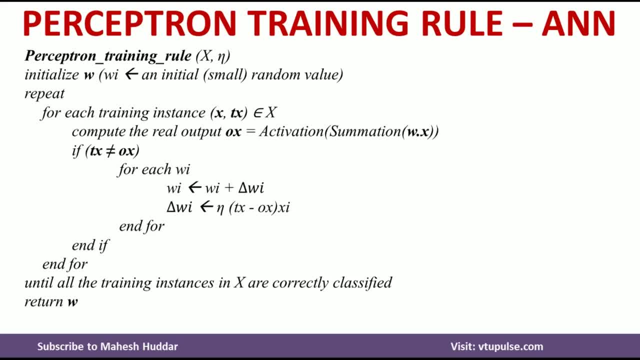 First we initialise the weight vector to a small random value For each training instance. we repeat these steps. The training instance contain x and the target. First we compute the real output, ox, by applying the summation and then the activation function. If the target output is not equivalent to the actual output for each weight, we perform these two steps, that is, we modify the weights using these two equations.